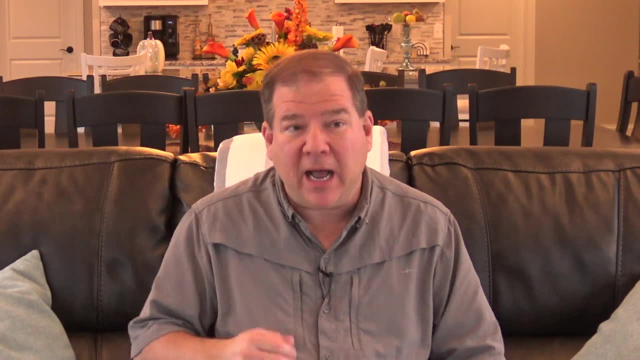 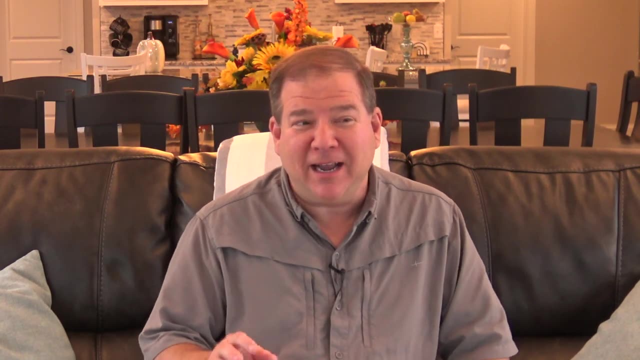 When I first got into IT back in 1989, I started working with Cisco's very first router. It was an old Cisco AGS Plus router. Well, actually back in those days, instead of calling them a router, they called them browsers. 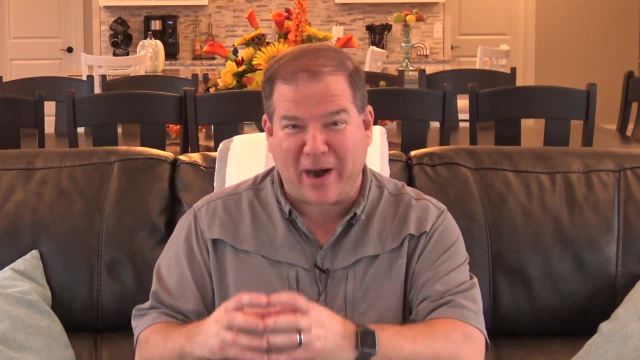 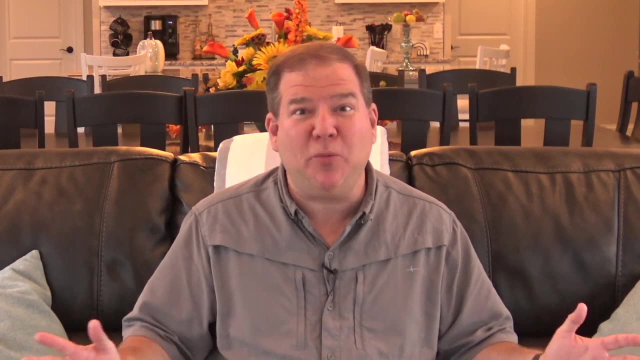 Because this device was both a bridge and a router, so it was called a browser, But it's what you and I know as a router today. I loved working with it, but I was super confused about so many aspects of working with that box. I was confused about how to do subnetting and how. 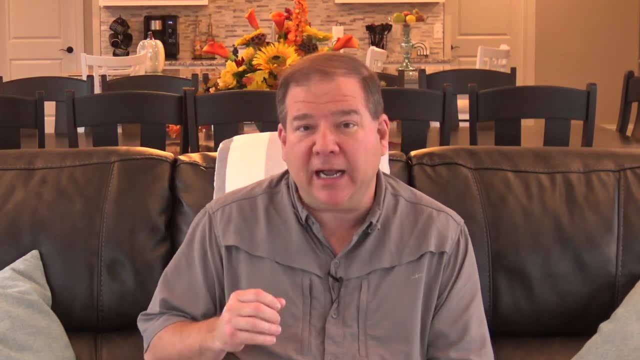 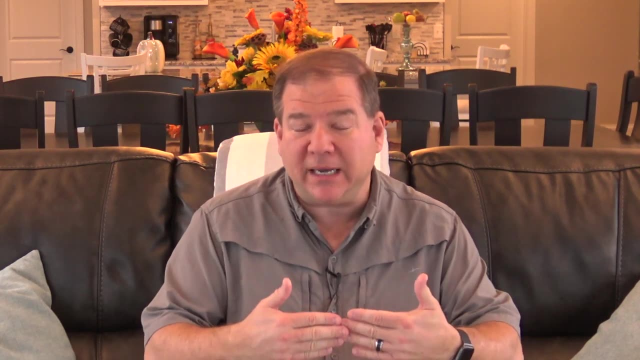 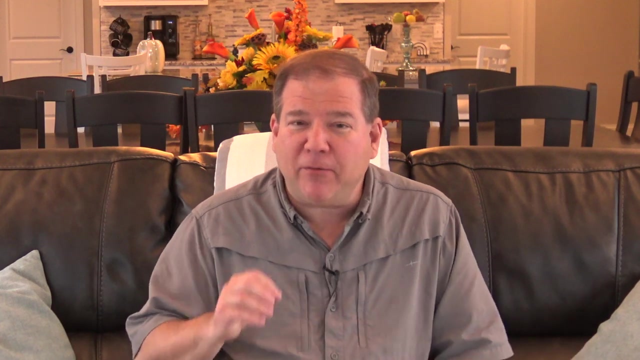 to do a lot of the configuration. but I was super fortunate. I had some great mentors that walked through that journey with me, gave me resources and eventually I got my CCNA certification And that changed my life. That was way back in 1998.. And from that point on I just started. 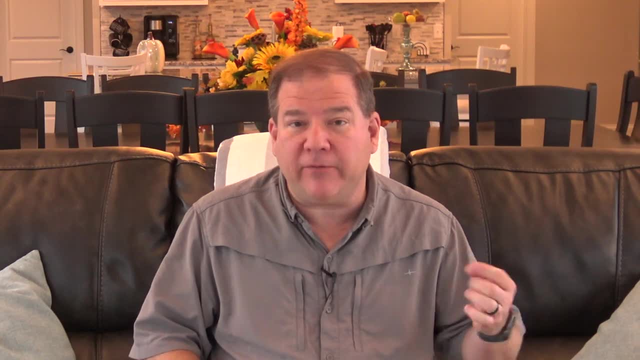 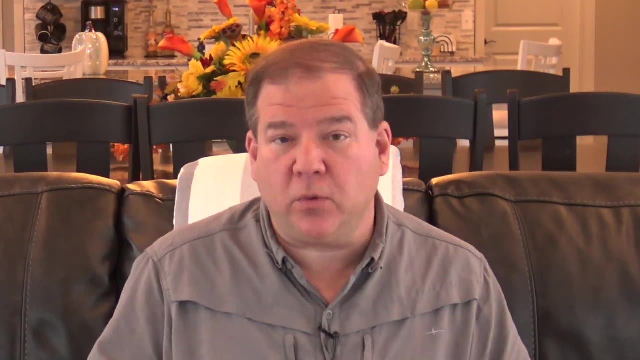 getting more and more certifications. Three years later I got my first CCA. Years. after that I got a second CCA And my real-world experience includes teaching for Cisco Learning Partners for about 14 years And I used to be a network designer- one of five network designers down. 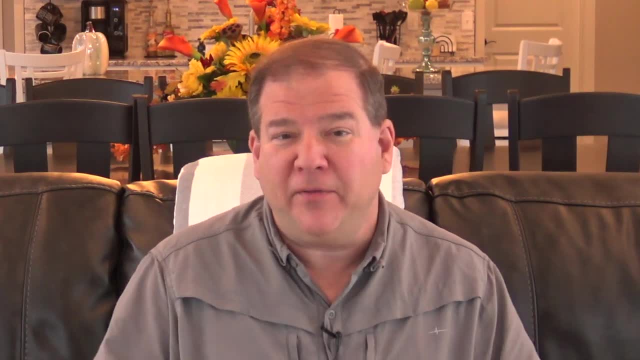 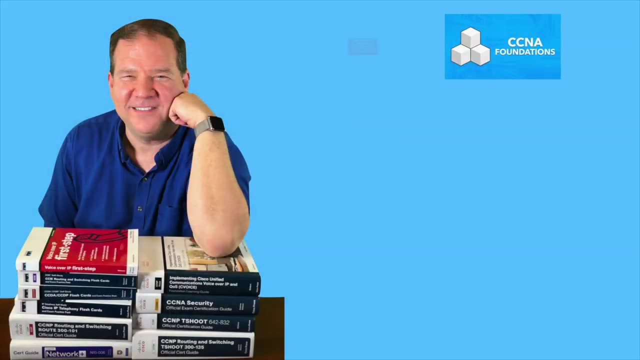 at Walt Disney World in Florida. I designed the network that tied together the Magic Kingdom with Epcot and the Animal Kingdom and the studios and a lot of the other things And I was able to get a lot of the resources And I've created a bunch of books. I've done a lot of video courses And 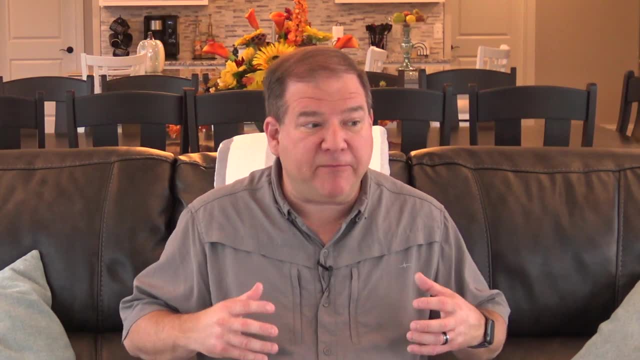 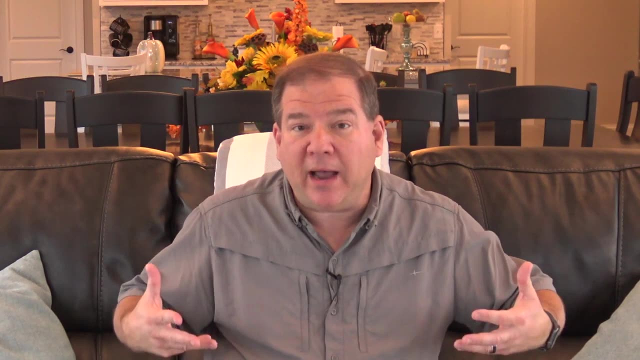 what I want to accomplish for you in this CCNA mini course is to see if this stuff resonates for you. I want to give you a sampler platter of a lot of different CCNA content and see if you have the eye-opening experience, like I did, and realize that this is your future. This is 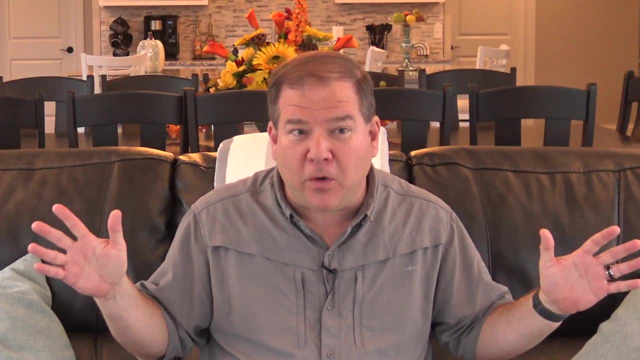 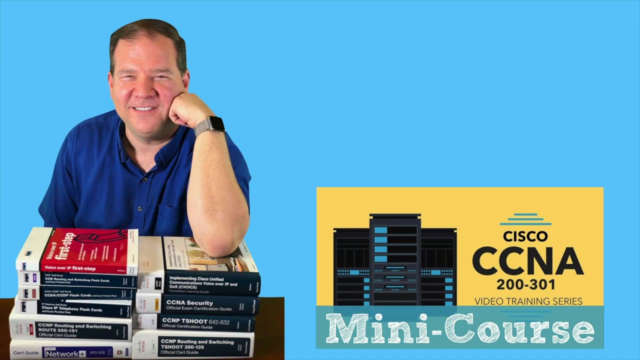 where you want to go all in. If it's not, that's totally cool, But I thought this would be a good way for you to test the waters going through this mini course. So here's the game plan as we go through this mini course. I'm going to give you some sample content over a series of days from: 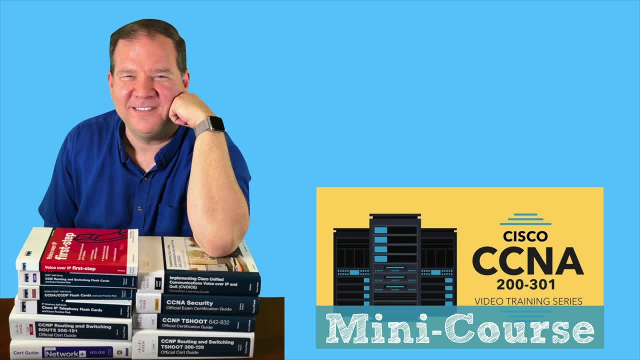 different areas of the CCNA curriculum. Specifically, we're going to be taking a look at quality of service, the spanning tree protocol and wireless standards. And if you're concerned that you might not have the background to go into these studies, don't worry, I'm going to keep these topics very. 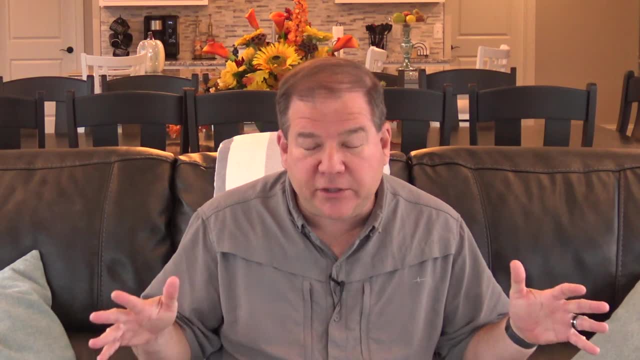 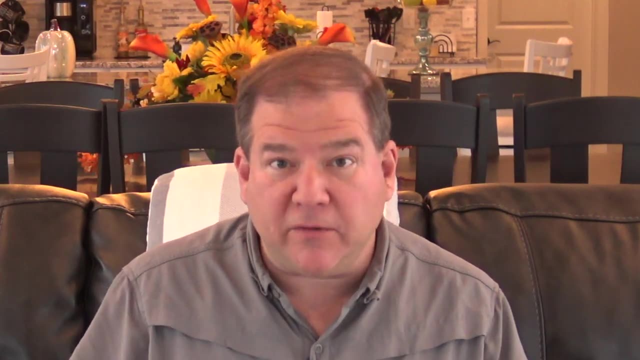 conceptual in these videos. We're not going to be getting into a lot of configuration. I just want to see if this stuff resonates with you or not. Now let's get started in this video by checking out what quality of service is all about. Then, after I show you that clip from our CCNA course, 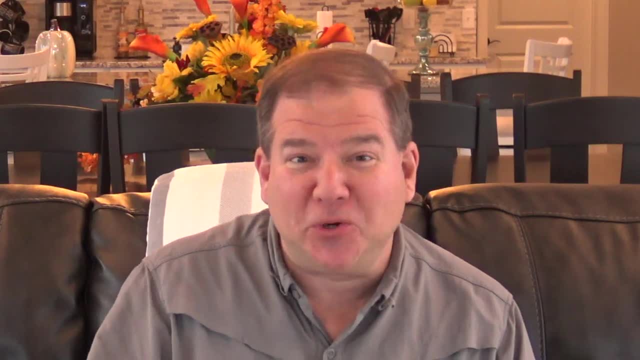 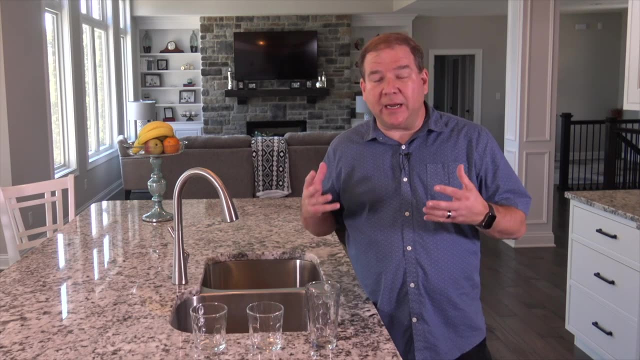 we'll come back, have a brief chat and I'll give you your next steps. Enjoy the video. In this lesson, we want to consider quality of service, And quality of service is really a collection of features that we can use to protect certain traffic from other types of traffic. We 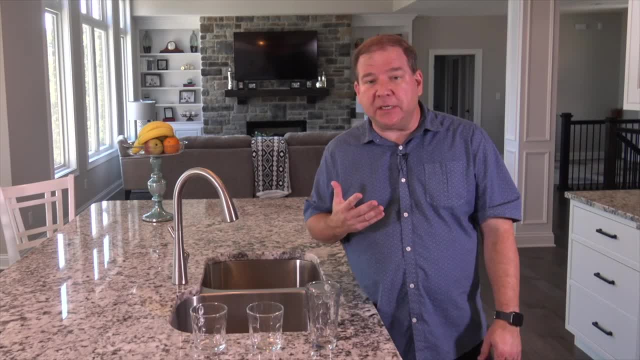 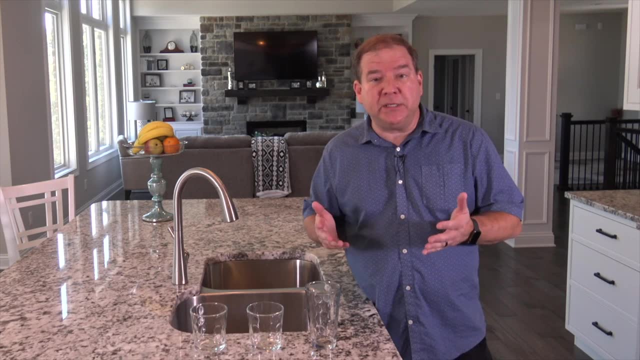 can give preferential treatment to specific traffic types based on our business needs. And while there are lots of QoS mechanisms, consider this simple example of how we protect voice on a really busy network. Imagine we had a router that goes out to the wide area. 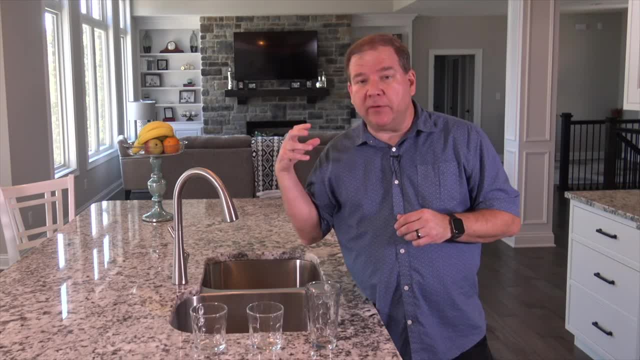 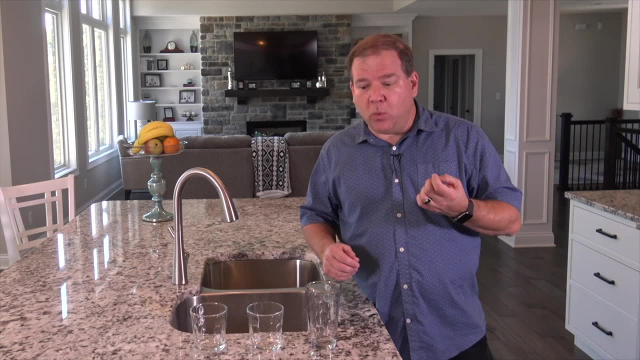 network. Now we're coming into that router at a gig rate. We're coming in from the local area network, But we're going out to the WAN at only 100 megabits per second. one-tenth of the rate. Well, that's a big speed mismatch. So traffic is going to be coming into the router faster than 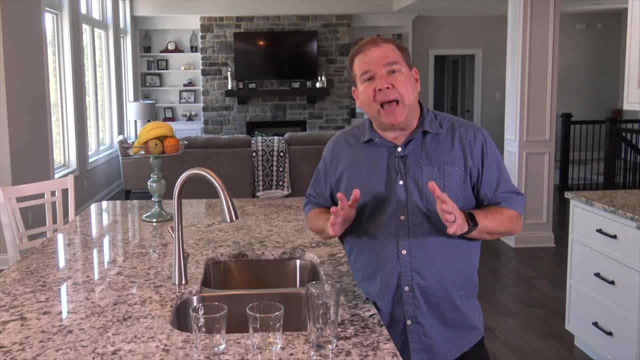 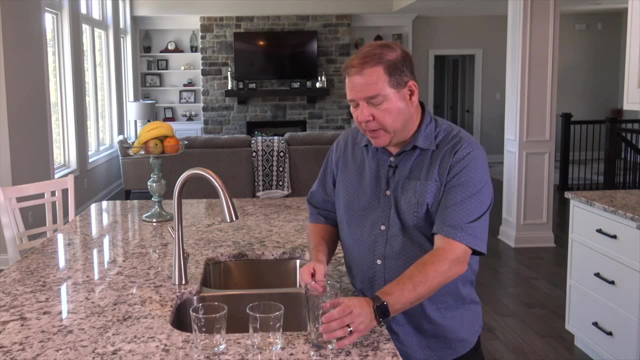 the router can send it out. So what does the router do? The router is going to allocate some memory called a buffer or a queue, and it's going to temporarily store those packets in that queue. Imagine that we had a queue the size of this. This is going to represent our queue and the 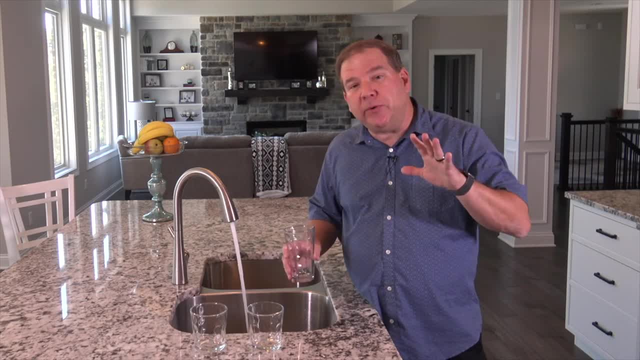 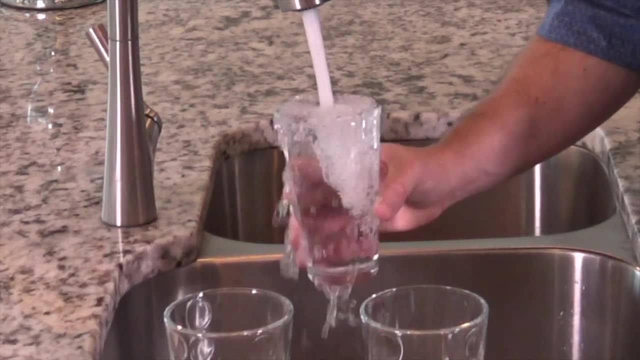 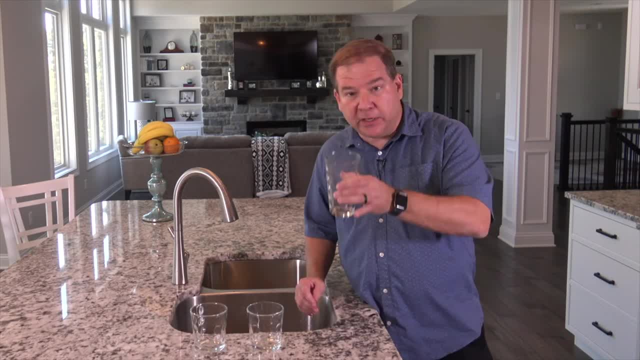 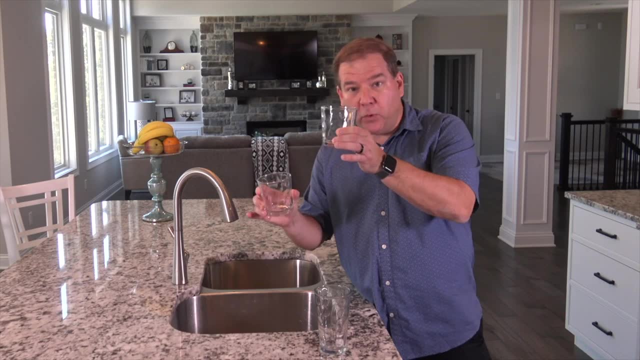 what if we did queue separation? Let's say that we took this queue on the interface and we divided it into smaller queues, but we're going to put voice in one and we'll put everything else in the other, And we've still got our big data burst on the network. Well, we've got a little bit of voice. 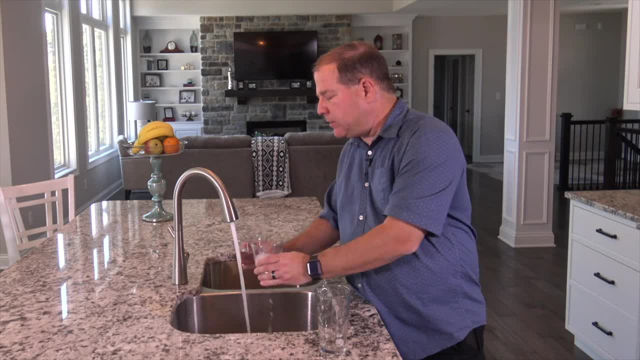 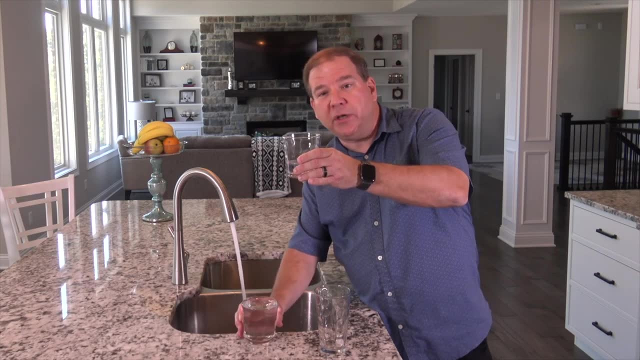 traffic and we've got lots and lots and lots of data traffic and a little bit more voice, a little bit more data And eventually the data queue is going to start to overflow. Meanwhile, our voice queue is protected. We're not dropping voice packets, even though we are dropping data packets. 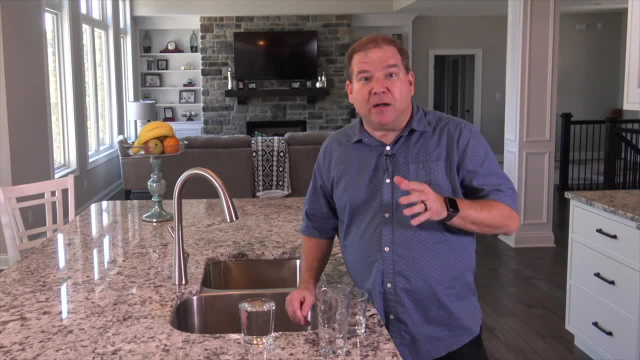 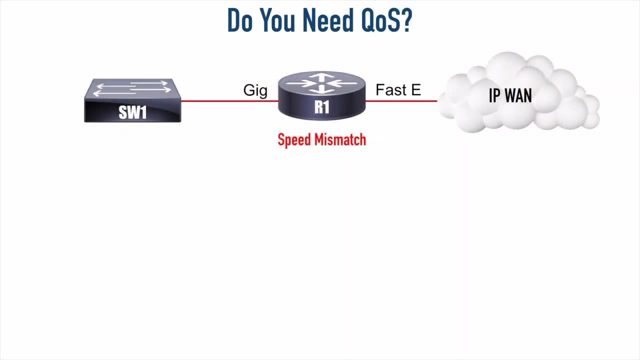 That's just one example of what quality of service can do for us. Now join me in our next video as QoS fundamentals. Let's consider the fundamentals of quality of service, or QoS. The best definition I've ever heard of QoS is that QoS is really managed unfairness, If you think about that. for 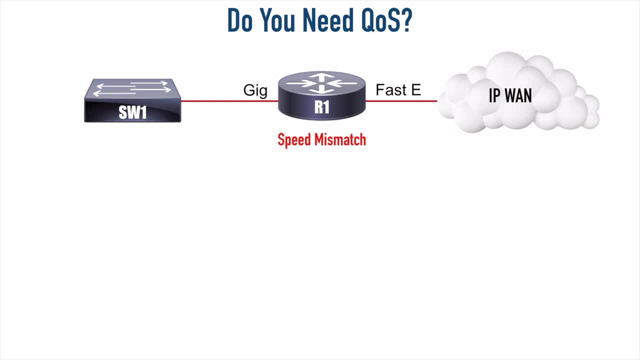 a second. that's exactly what it is. We're being unfair to certain types of traffic so that we can give higher priority to other types of traffic. but we're in control. We get to manage who we give preferential treatment to. So it's managed unfairness. But why do we need it or when do we? 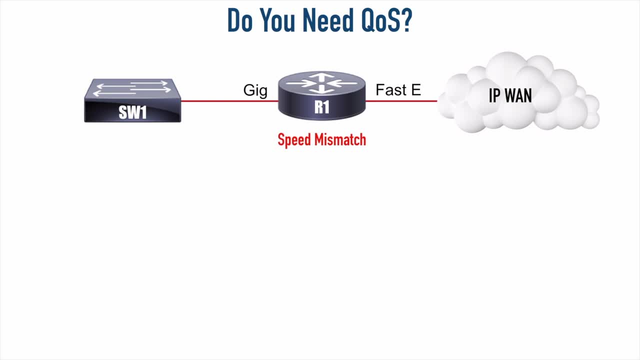 need it. Let's think about this example. Here we're coming into router R1 at a gig rate but we're leaving at a fast Ethernet rate going out to the IP WAN And even though those are both fairly high speed interfaces, there's a 10 to 1 speed mismatch there. We could be coming into router R1 from. 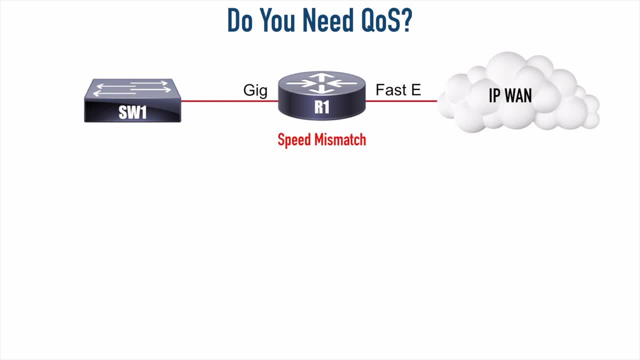 switch SW1 at gig rates and we're trying to go out at one tenth of that rate. That's not going to work very well. That's where we might need to do quality of service, to prioritize who gets to go first And if we have to drop somebody, who's going to get dropped. 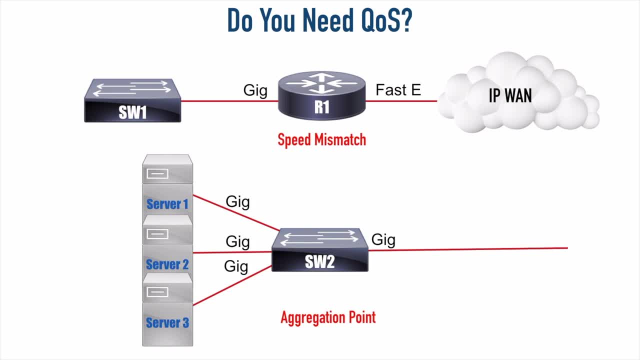 Another place where we could have a need for quality of service is when we have an aggregation point. Here. switch SW2 has exclusively gig interfaces And we might think that this is a high speed network and no need for quality of service here. But if we have lots of servers, 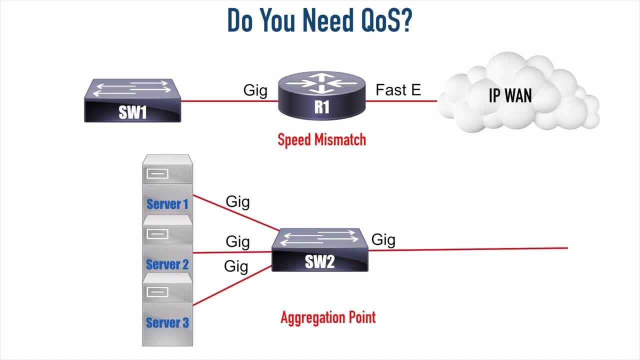 coming into switch SW2 and trying to leave over that single gig link. we could be coming into the switch at multi gig rates and trying to leave at just one gigabit per second. That's not going to work very well And a huge point to understand about quality of service is that, while it can help, 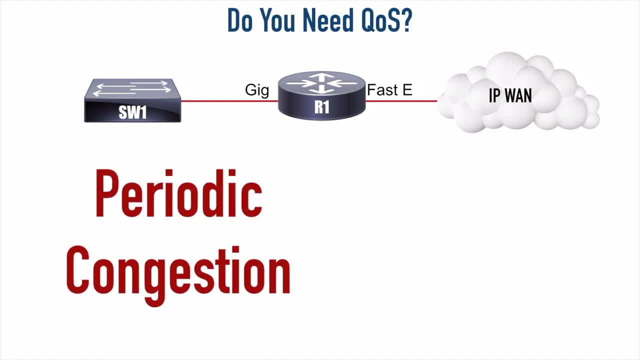 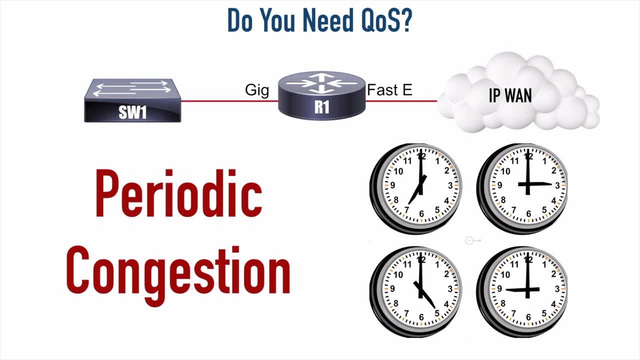 us out in situations like this. it's good for periodic congestion. If we're congested 24-7, then we need more bandwidth. But if we just have periodic times of congestion, maybe first thing of the morning, maybe first thing in the morning when everybody is powering- 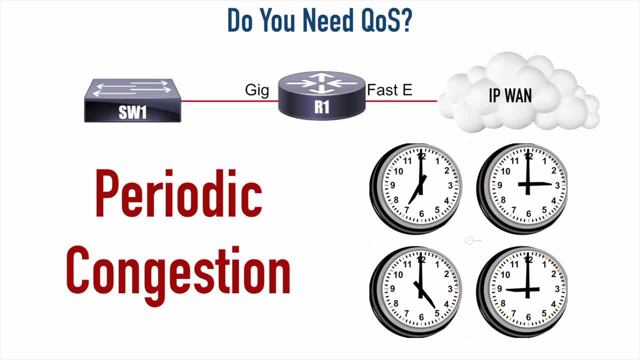 their devices on, maybe overnight, when there's a network backup going on. If there's just periodic times, then yeah, quality of service might come to the rescue. But if we're congested all the time we probably need more bandwidth. And we can break quality of service down into three different. 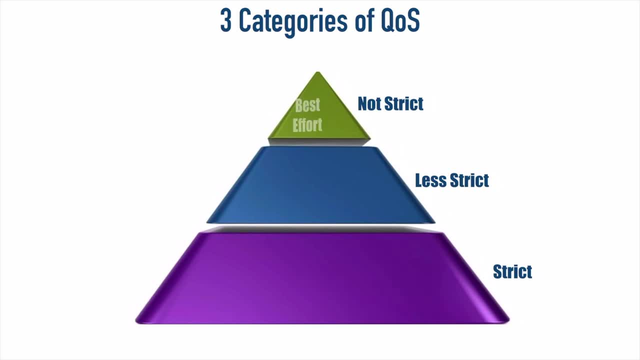 categories. The first category, that's not strict at all, is called just best effort. This is FIFO. first in, first out. I hesitate to even say that this is a category of quality of service, because we're not doing any reordering of packets, We're not giving any prioritized treatment. 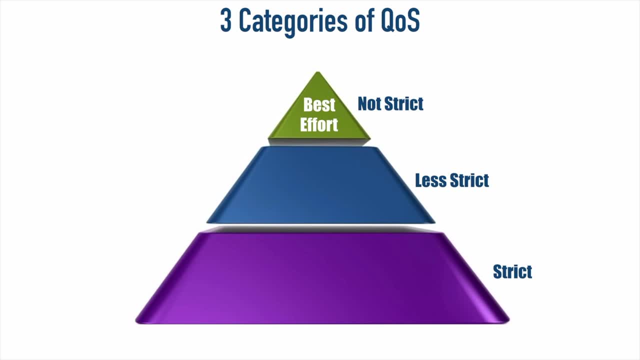 It's just the first packet that comes in is the first packet that gets sent out, And then we have strict and less strict categories of quality of service. The less strict is what we mainly focus on. This is mainly what's used in the real world And it's called diff serve. 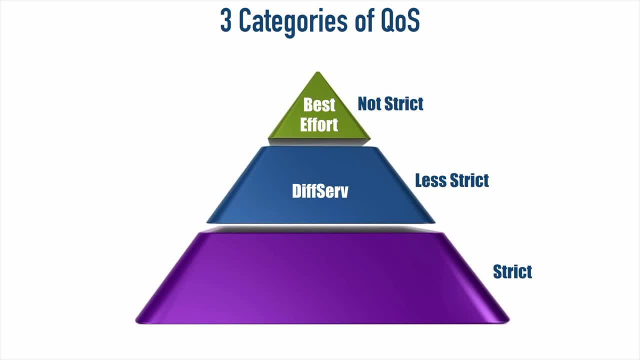 That stands for differentiated services. We are differentiating between different packet flows and treating those different traffic flows differently. The strict option is called int serve for integrated services. Here's where we have something like RSVP, the resource reservation protocol- where we do make a hard and fast reservation for a type of traffic And we don't 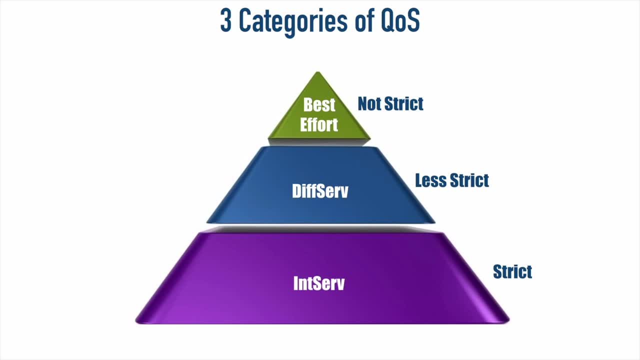 give that bandwidth up until that reservation is released With the less strict option we share. If a type of traffic doesn't need the bandwidth at the moment, we can let somebody else use it. This is typically what we're going to be using, And there are several quality of service tools. 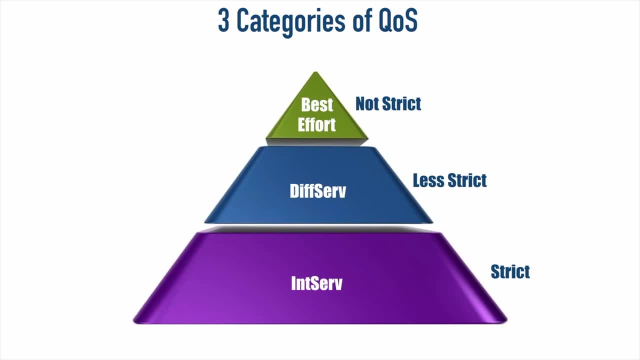 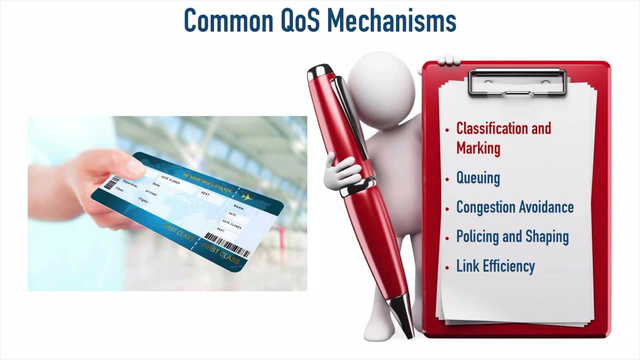 that we can turn on within Cisco iOS, But at a high level. let's consider these different quality of service mechanisms. The first is classification and marking, And Cisco recommends that we classify and mark our traffic as close to the source as possible. As an analogy, consider: 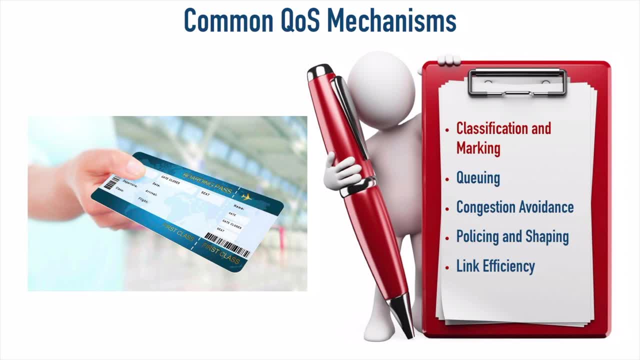 getting on an airline Now. personally, I fly Delta primarily, but I've still not received any silver medal or whatever. that level is where you get to get on the plane early. I'm not there yet, I'm working on it, But can you imagine when the day comes I finally get sky priority or whatever? 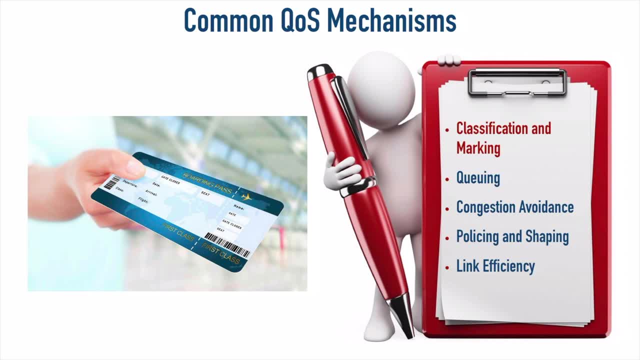 they call it and I go up to the gate agent and they say: well, Mr Wallace, before you can get on the plane, can you show us the boarding pass from the time you went to Orlando and Chicago and San Jose and Austin? That's not very efficient, is it? If I have to prove myself every time I get. 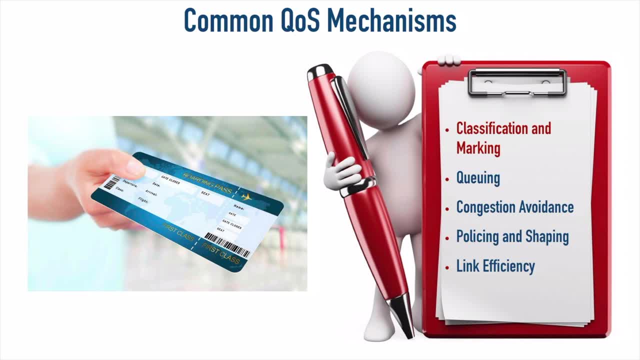 on the plane. So what do they do? They put a marking. They actually put a marking on the boarding pass that says something like sky priority And, as a result, they can very quickly, very efficiently, look at that marking and know that, yeah, I get to get on first, I have priority. 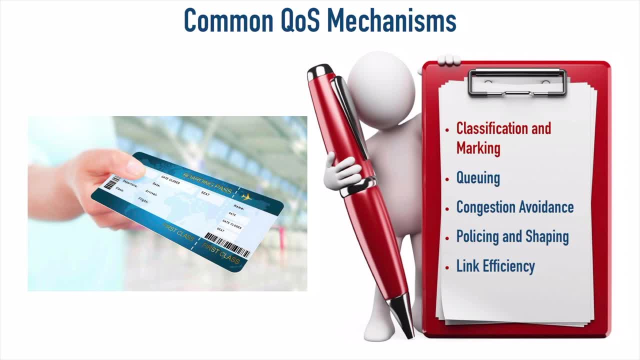 treatment. It's the same thing with our quality of service mechanisms. If we recognize the type of traffic early on in its travel, we can give it a marking, And we're going to be talking about some of those different types of markings in an upcoming video. But if we mark our traffic early, 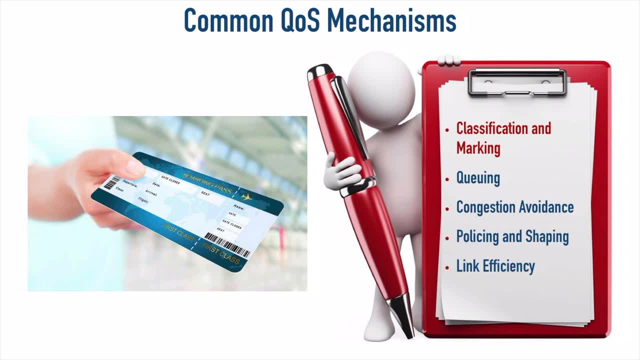 on. then the next route or the next switch can very quickly, very efficiently, very efficiently look at that marking and make a decision, like a forwarding decision or dropping decision, based on that marking. But marking traffic by itself doesn't really alter the behavior of the traffic. 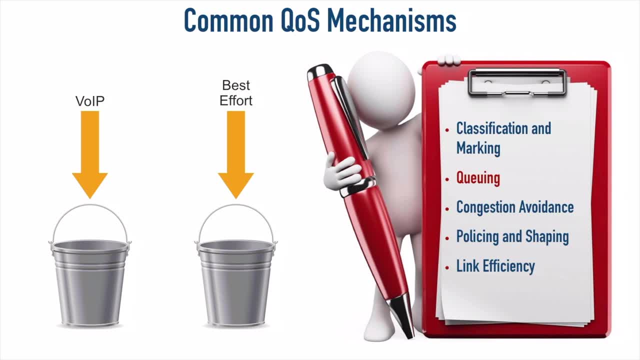 We have to have some other mechanism to look at that marking and do something with it. For example, think about queuing. Queuing is also known as congestion management, If you think about a router and we're coming into a router at a high speed and we're trying. 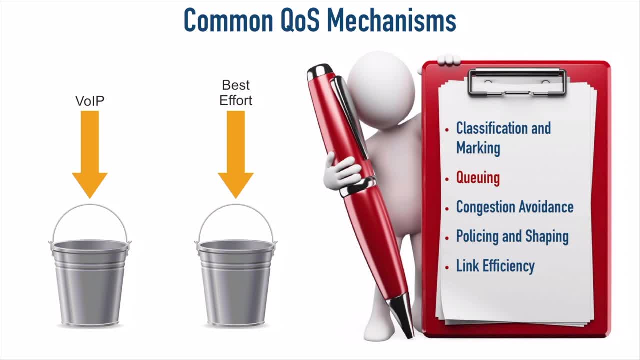 to leave at a lower speed. well, that exit interface, that egress interface, has a buffer- Sometimes we call it a queue- And that buffer, that queue, has a finite capacity. It's able to store so many packets in the queue until, hopefully, Bain with demand dies down and 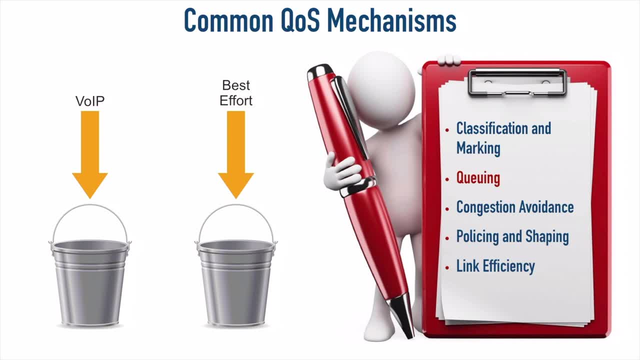 we'll be able to take packets out of the queue and send them on their way. But if we just have that one queue space and all sorts of traffic are piling into that queue, when that queue fills up you could think of it like a bucket. When that queue fills to capacity, it's going to start to. 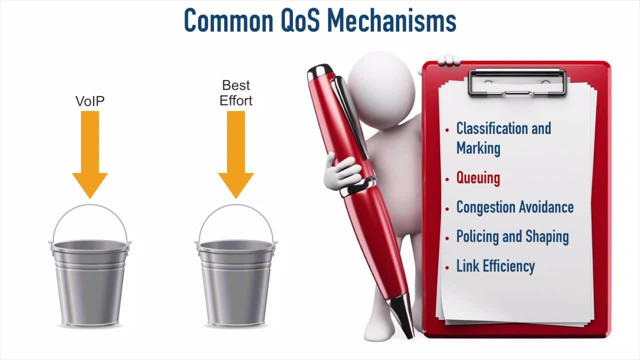 overflow, just like water overflowing in a bucket. Something we could do to help protect our sensitive or important traffic is to take that queue space and divide it up into sub-queues. As a simple example, that's what I've done here. I've got one voice over IP queue or a bucket and I've got a best effort: bucket for everybody else. 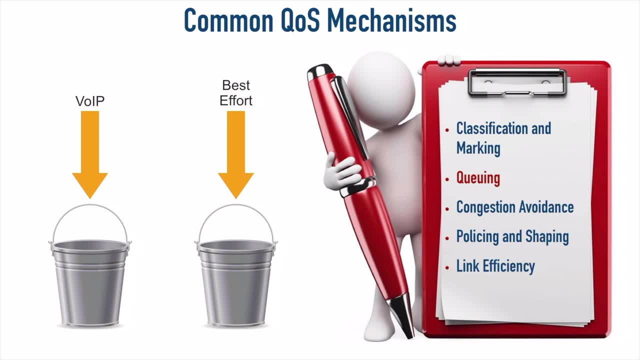 Well, let's say that we do have a big burst of data on the network right now and we've got traffic flowing in and that best effort bucket is filling up and it's starting to overflow. We're dropping packets, Meanwhile the packets 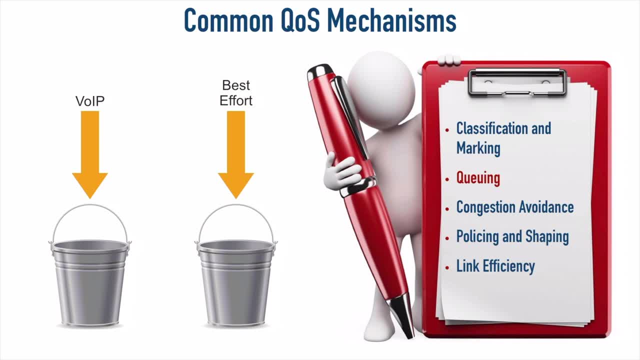 that we've recognized as voice over IP packets. they're just going into the voice over IP bucket. It's nowhere near capacity. We're not overflowing there and we can send traffic in that bucket first. So just by doing this basic queue separation we're already giving a priority. 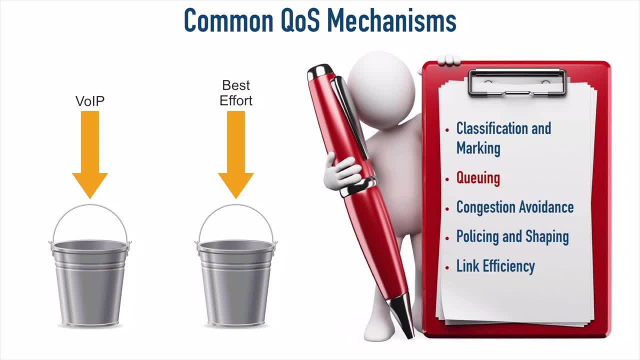 treatment to voice over IP And we said queuing was congestion management. Well, on the flip side of that, we have congestion avoidance. Congestion avoidance means we're trying to prevent a queue from ever filling to capacity to begin with, And what we're doing is 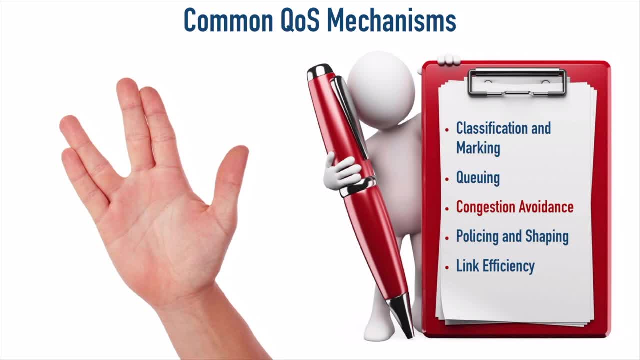 keeping an eye on how many packets we have in a queue, And we could keep an eye on each of the sub queues if we wanted to do it that way, And after we exceed a certain threshold we can say: I'm getting a little bit nervous, This queue is starting to fill up and some really bad things. 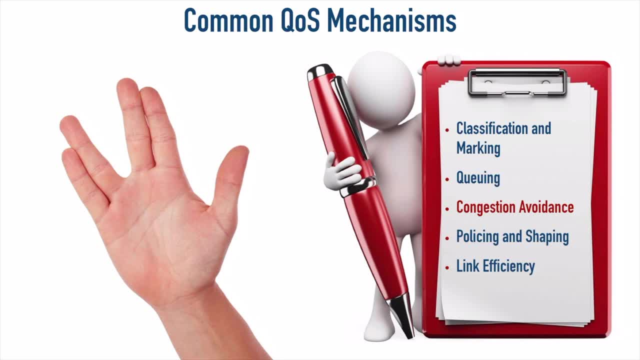 happen if the queue fills up. For one thing, all the traffic coming into the queue gets dropped if the queue is at capacity. But it's even more insidious than that If you think about the way TCP works. TCP has a slug of traffic coming into the queue. And if you think about the way TCP works, 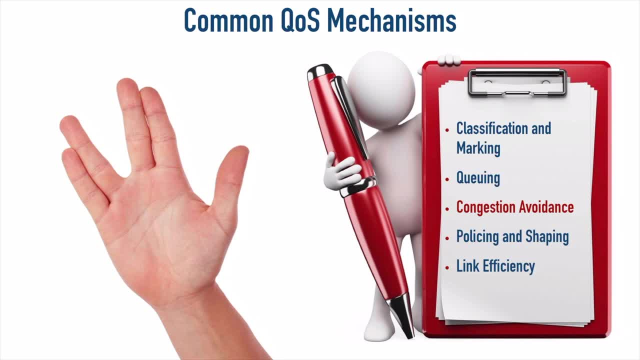 when we first do that TCP three-way handshake and we set up a connection between a couple of devices, that first device might send one segment And if it was received successfully, the recipient's going to send an acknowledgement saying: got it, send me the next segment. 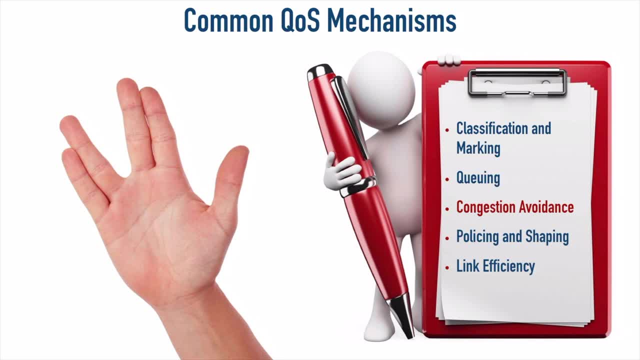 And we say: oh, that worked, I'll send two segments this time. Then, when those are acknowledged, we'll send four segments and eight, 16,, 32,, 64,, 128, and so on. We keep doubling our window size. 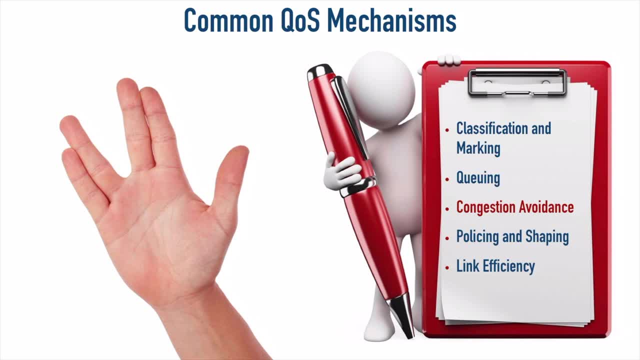 which makes for more efficient communication. We're spending less time waiting for an acknowledgement. Well, if something happens, maybe a packet gets dropped and the acknowledgement comes back saying: all right, give me segment number 5,025.. And we thought we already sent that. We realize we're sending too aggressively. 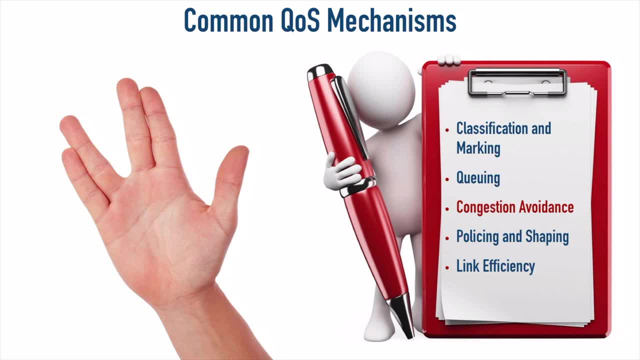 Something's wrong. We need to slow down, We need to reduce our window size and we'll start sending a lower number of segments. And while that's just normal for TCP, it's not a big deal If a queue fills to capacity, we're going to have to send a segment. number five, six, seven. 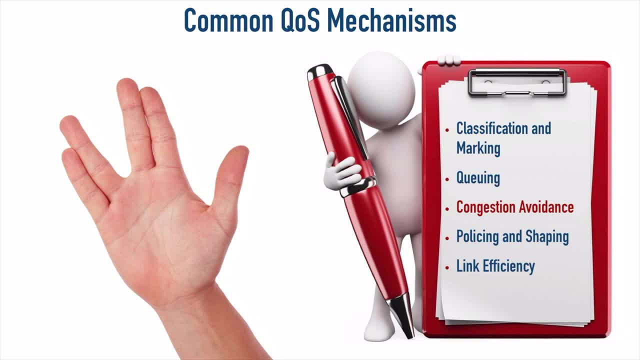 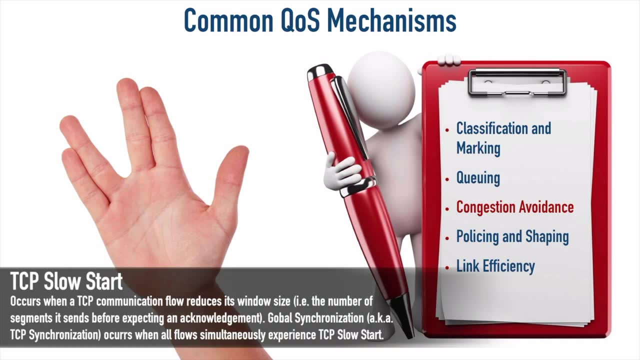 every TCP flow going into that queue is simultaneously going to start dropping packets and reduce their window size. And when a single flow does that, it's called TCP slow start. When everybody does it, it's called global synchronization, or sometimes it's called 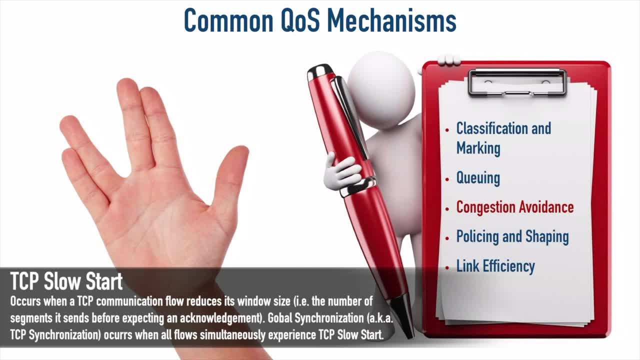 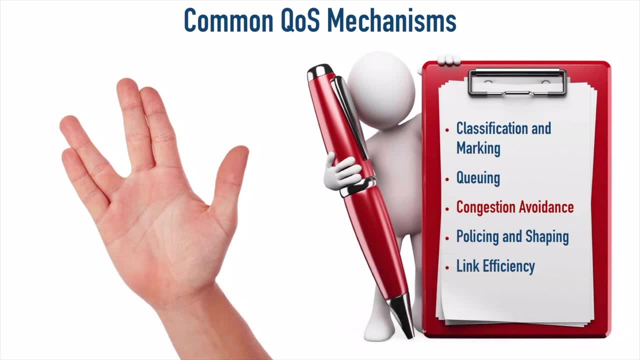 TCP synchronization And it results in a very inefficient use of bandwidth. To prevent that type of thing from happening, we can keep an eye on traffic And if we start exceeding a certain level we can discard that traffic. And the reason I have the 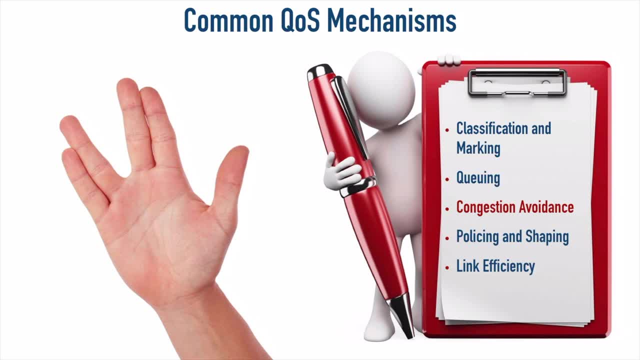 Vulcan live long and prosper. symbol on the screen is the congestion avoidance mechanism that we use reminds me a lot of my favorite Star Trek movie. It's Star Trek two, the wrath of Khan. Remember Ricardo Montalban? he was Khan and he was about to blow up the enterprise, but the warp drive was. 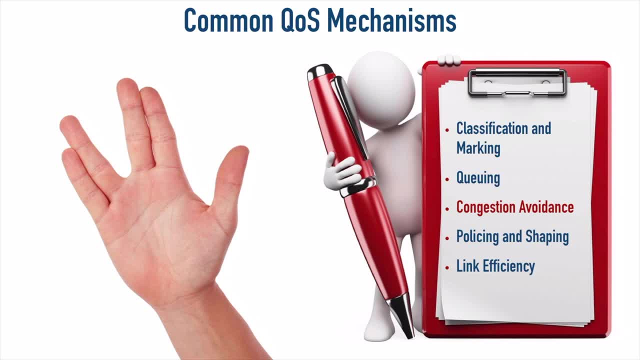 damaged and they couldn't get away. So spot goes down into main engineering and he fixes the warp drive. but he's exposed to all this radiation and he's blinded by it. And then Kurt comes down to see what's going on And Kurt goes. 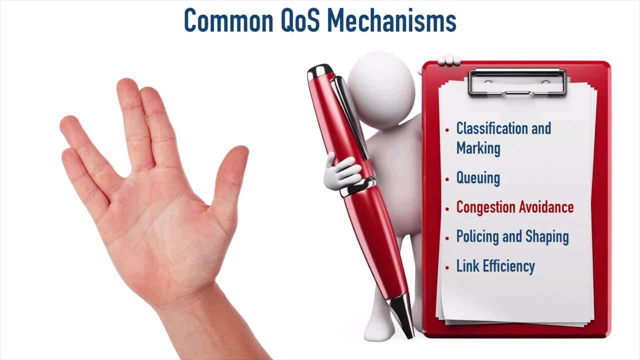 up to the glass and he says Spock. and Spock comes up to the glass and he says: don't grieve, admiral, It's logical. And I paraphrase: He said: the good of the many outweighs the good of the few. And Kirk says: 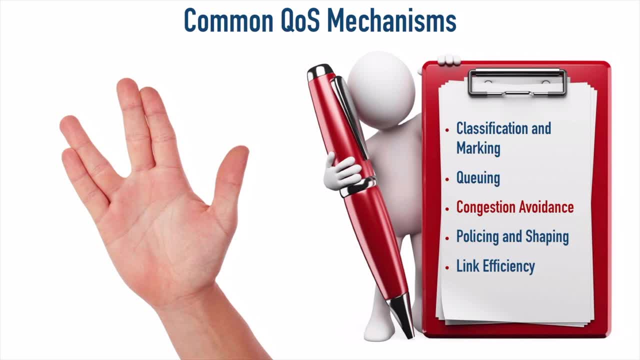 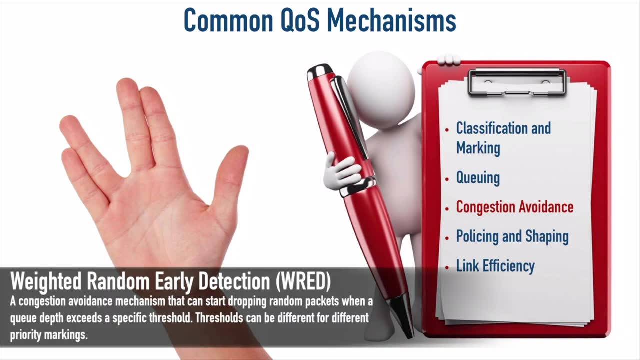 we're the one. And that's really what our congestion avoidance mechanism is doing: It's sacrificing the few for the good of the many. It's throwing away some packets so that other packets don't have to suffer global synchronization or packet drops. And the mechanism we're going to be using in our Cisco 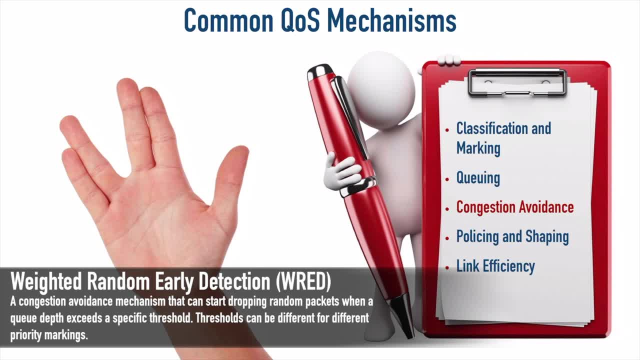 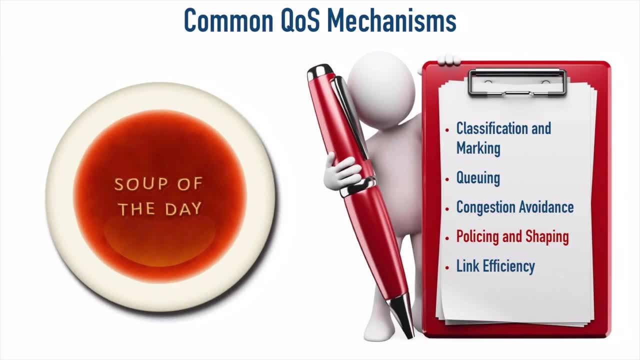 routers is called a weighted random early detection WRED. Our next category of quality of service mechanisms is a traffic conditioner, And we have a couple of types of traffic conditioners. We have a policer and a shaper. Policing and shaping: both have the same purpose in life. 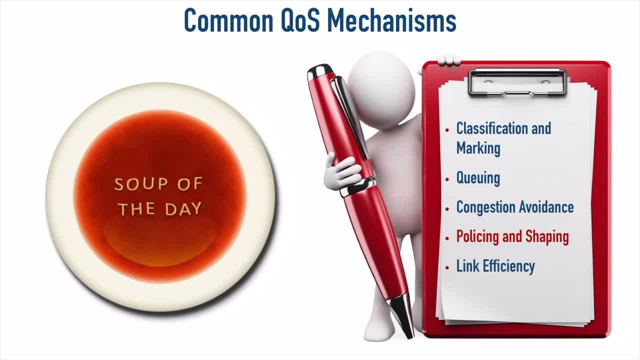 and that's to prevent traffic from being sent too aggressively, too rapidly, While something like queuing is guaranteeing a minimum amount of bandwidth that we can send policing and shaping, they're setting maximum amount of bandwidth that we can send Policing and shaping. they're setting maximum amount of bandwidth that we can send. 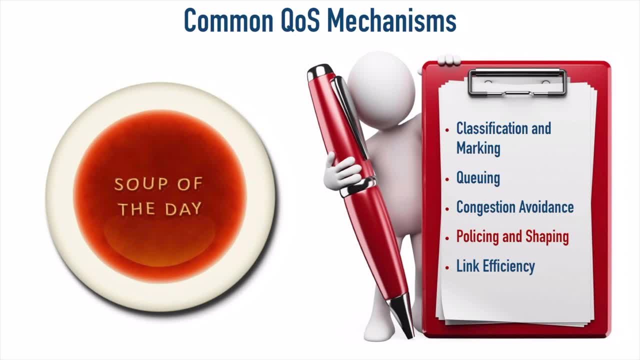 Policing and shaping. they're setting maximum amount of bandwidth that we can send. It's setting a speed limit on our traffic And Policing is typically more harsh. Policing says by default: if you violate this rate that I've set, then I'm going to drop you. 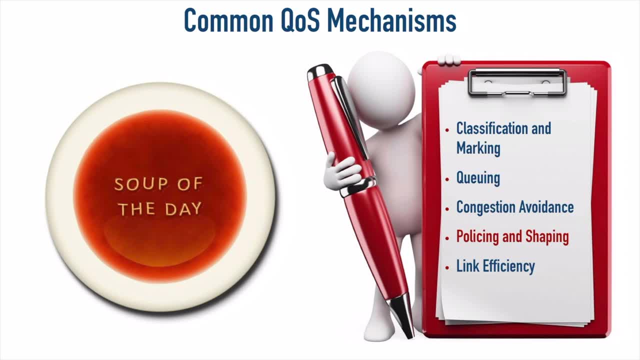 And the reason I have a bowl of soup on screen is that it reminds me of that Seinfeld episode where, if you don't order soup correctly, the guy says no soup for you. come back one week. That's what policing is doing. 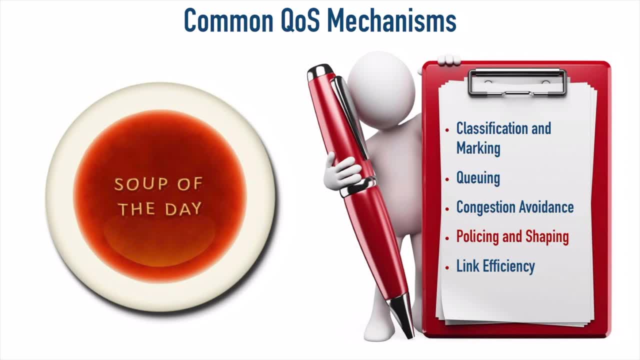 If we exceed the speed limit, the router or switch can say: no bandwidth for you, come back. Literally come back back, meaning that we have to retransmit that traffic because we've been dropped. Shaping, though, is a kinder and gentler approach to setting a speed limit. 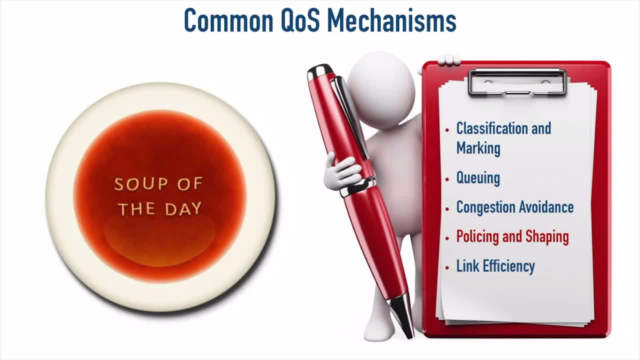 Shaping says: I'm so sorry, I don't have enough bandwidth to send you at the moment. but don't go anywhere. Let me just have you stay in this queue temporarily and then, when bandwidth does become available, you can come out of the queue and we'll send you on your way. 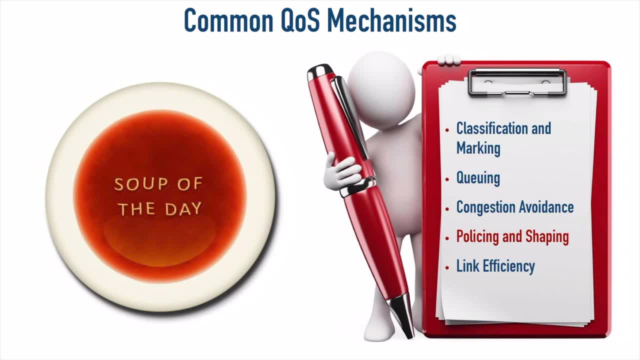 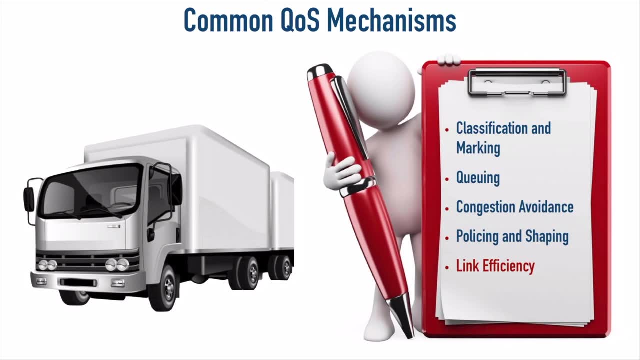 So shaping is going to delay traffic, while policing is going to drop traffic that exceeds the speed limit we set. And our final category of quality of service mechanisms is link efficiency And, honestly, this is not as important as it used to be. Link efficiency used to be a big deal when we were trying to make the most efficient. 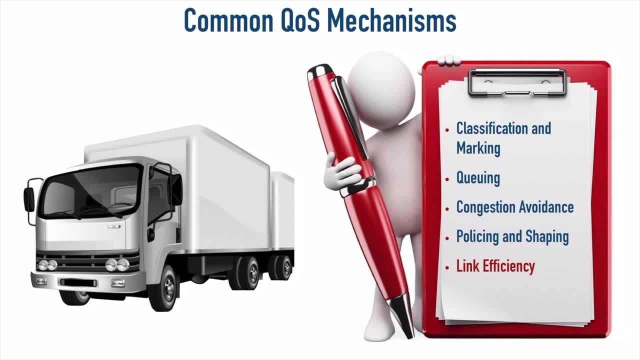 use of our link speeds on speeds that were less than 2 megabits per second or, in some cases, less than 768 kilobits per second. With today's high-speed networks, this is not the issue that it used to be. 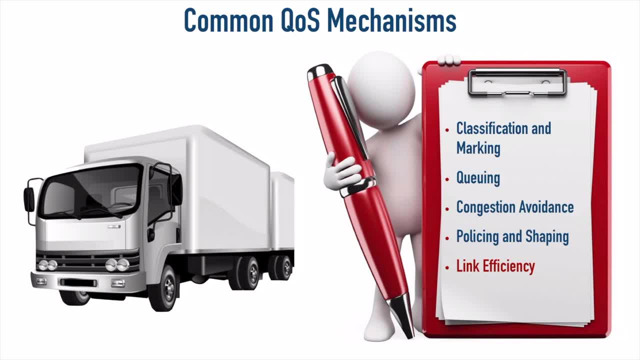 But for completion's sake I want you to know what it is. We've got a couple of primary types of link. One is compression, For example, think about voice. Voice is carried inside of an RTP, a real-time transport protocol packet. 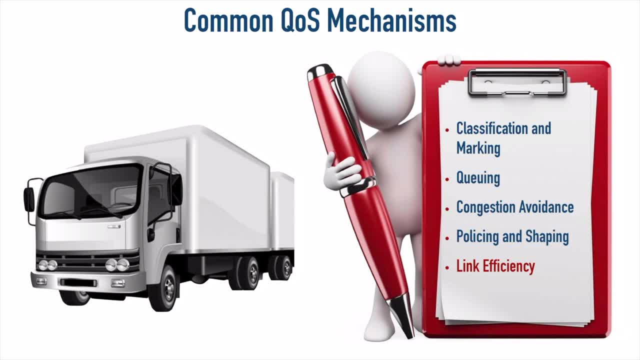 And if we add up the layer 3 and the layer 4 headers on that voice packet, that's 40 bytes in size. Now, depending on how we encode our voice, we might be using something called G.729 as our coder decoder, our codec. 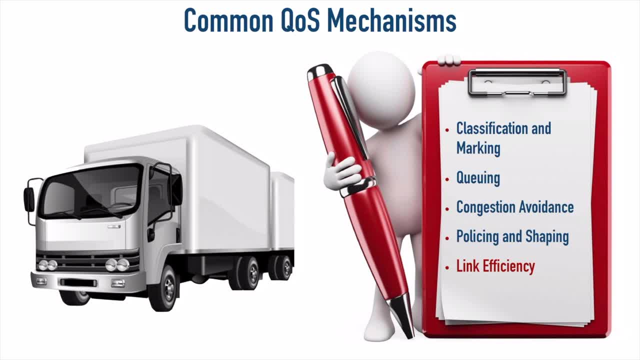 And with that, by default, our payload is only 20 bytes. We're only We're only carrying 20 bytes of voice, but we've got 40 bytes of header. That's a horrible ratio. So what we can do is something called RTP, header compression, where we're squeezing 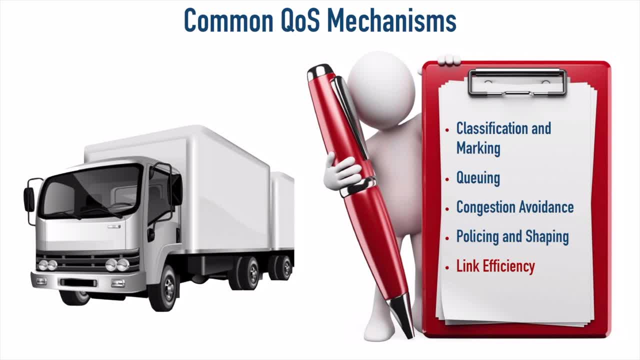 that header down logically from 40 bytes to only 2 or 4 bytes. Now, when I say we're squeezing it down, here's what's really happening. We're not really running a compression algorithm so much as we're caching the redundant information. 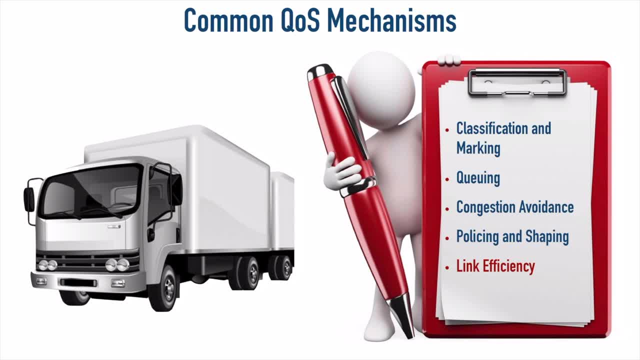 in the header. As a voice flow is going between a couple of routers, the routers can notice: hey, these headers have a lot in common. They've got the same source and destination IP addresses. They've got the same source and destination UDP port numbers. 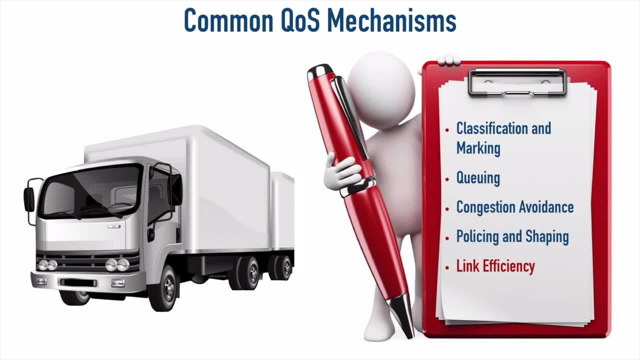 They've got the same RTP payload type. Why are we sending all this redundant information in the header of every single packet? Well, if we turn on RTP header compression, we don't. We make a copy of that information in the routers at each end of the link and we'll 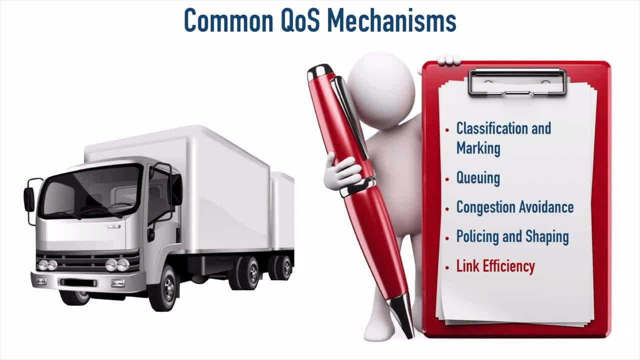 not send that redundant information. Instead, we'll just stick on a couple of bytes that can identify it as being a part of a particular conversation. Or there's an option to do a UDP checksum and that makes the header 4 bytes instead of 2 bytes. 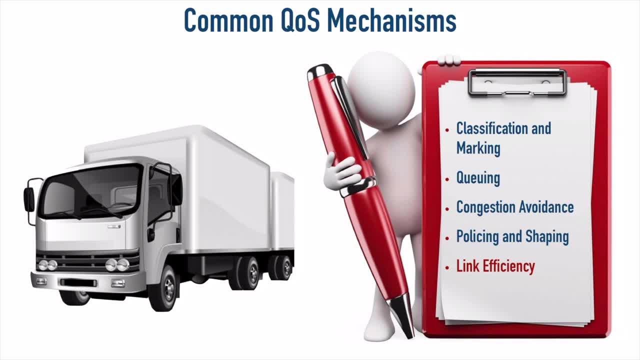 But typically in the Cisco world we're using a 2-byte header instead of a 4-byte header. That can save bandwidth and that's recommended for use when your link speed is less than 2 megabits per second. Another link efficiency mechanism is called link fragmentation and interleaving. 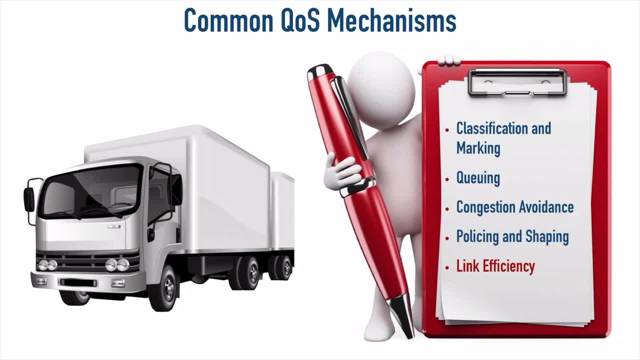 Consider the big tractor trailer that I have on screen. Imagine that we've got one, One of these big triple tractor trailers. Now, this one seems to only have a couple of trailers behind it, But in some places they're allowed to have on the roads, these triple tractor trailers. 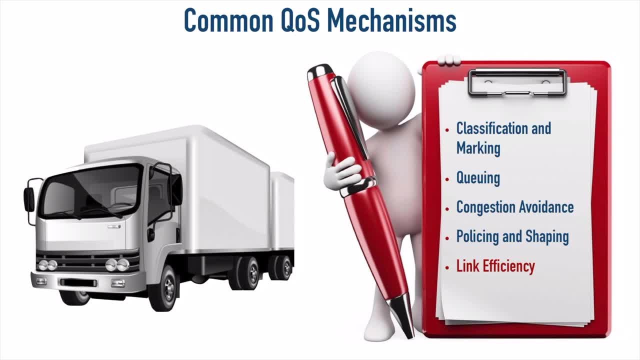 You've got the tractor in front and then the three trailers behind. Imagine that you're in a little tiny sports car and you're sitting behind one of these big triple tractor trailers at a traffic light. Well, imagine, the traffic light is like the interface on our router that we're trying. 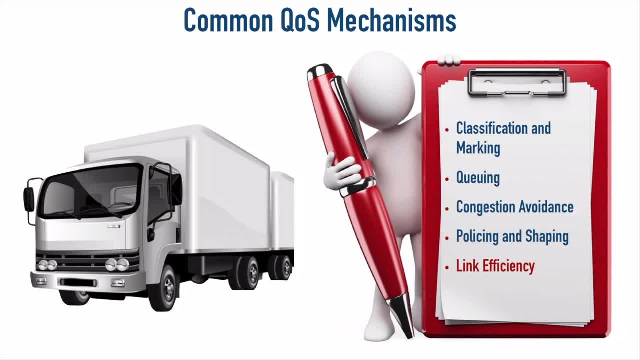 to get out of or trying to get through, And the big tractor trailer with this massive payload. That's a big data packet, maybe 1,500 bytes in size, And you in your little sports car you're like the voice packet kind of sitting there. 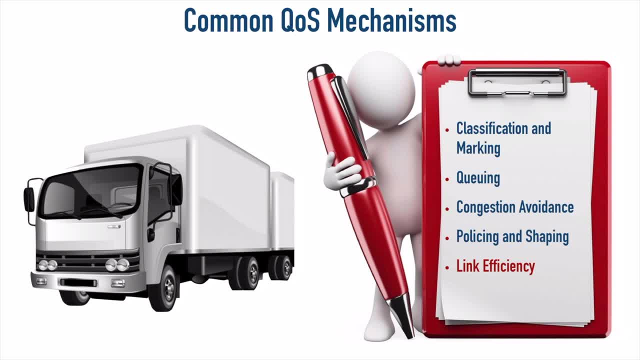 wanting to go through the intersection. Well, imagine the scene: The light turns green and the trailer starts to roll through the intersection and the first trailer goes through and the second trailer goes through. By the time the third trailer gets there, it's probably turned red again, and you don't. 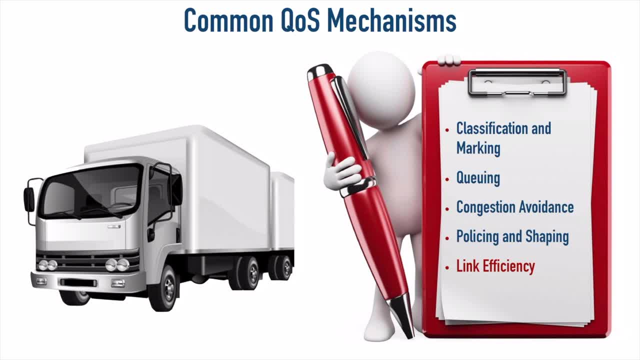 get to go through the intersection. yet That's a lot like it is with voice over IP traffic on slow speed interfaces. It can take a bit of time. It's a big data packet so long to get out of an interface that it's going to adversely. 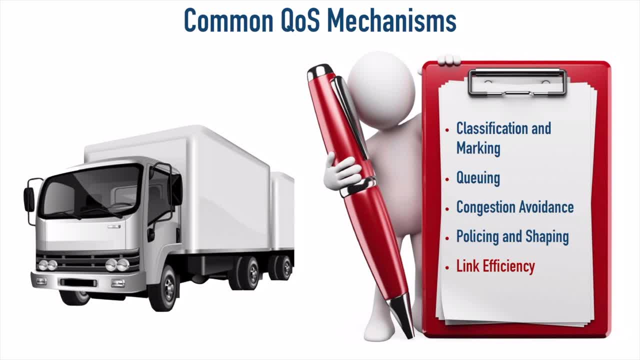 delay the voice traffic and it's going to sound bad. We're going to have bad voice quality due to too much delay. So what can we do? Well, what if we took that big tractor trailer and instead of having one tractor and then 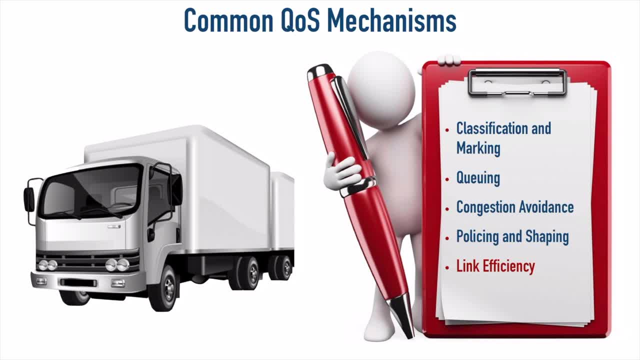 three trailers. what if we put each trailer behind its own tractor? Now we've got three separate vehicles on the road and we, in our little sports car, we could weave in and out. We're nimble, We're agile, We could get ahead of some of that traffic. 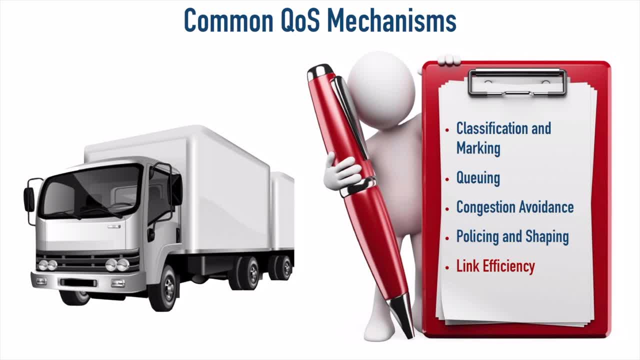 We could pass one or two of those tractor trailers and get through the intersection sooner. It's the same thing with our voice over IP traffic. If we did link, fragmentation and interleaving, we could take that big data packet and bust it up And then, just like we're shuffling a deck of cards, we could shuffle in the little tiny. 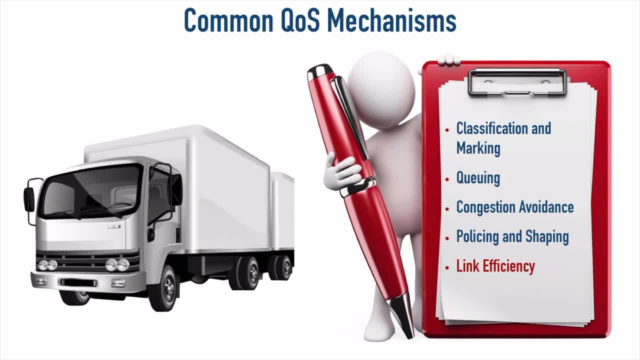 voice packets in amongst the now fragmented data packets and, as a result, the voice traffic gets through the interface sooner. All right, that's an overview of what is quality of service. why do we need quality of service and some of the different quality of service mechanisms out there? 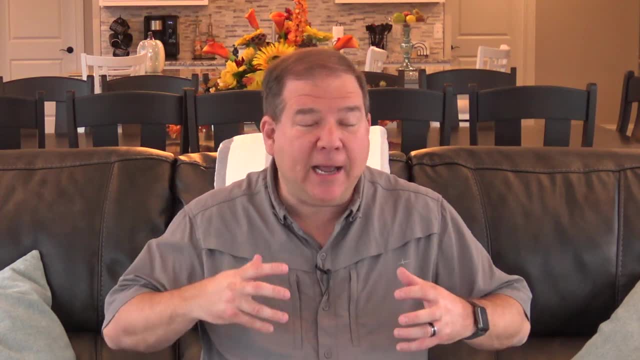 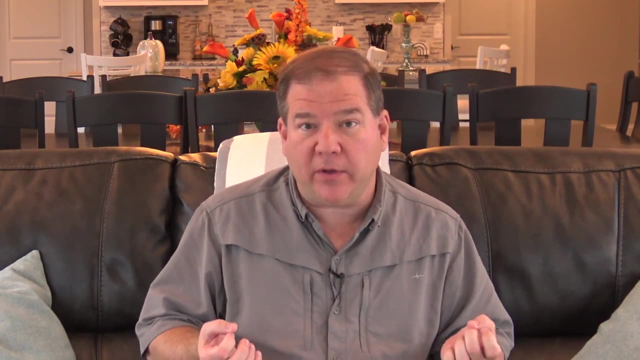 Well, I hope you enjoyed that training on quality of service And to help that information stick, here's my challenge to you. I want you to write in the comments area down below one big takeaway that you got from that QoS training. That's going to help it stay in your mind and you're also going to be able to review. 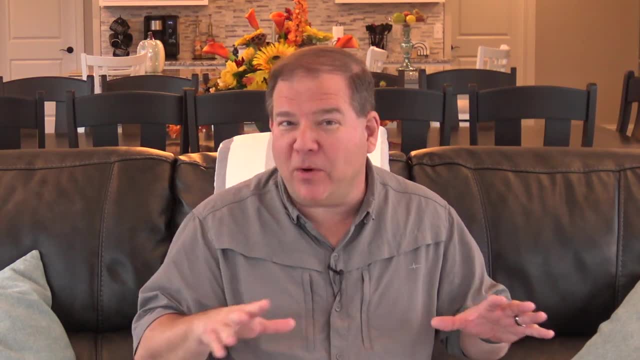 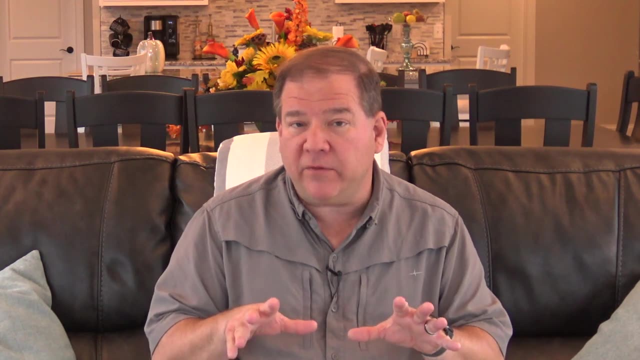 what we talked about by seeing what other people commented as they were saying what their big takeaway was from the video. And, by the way, since this is the first video in the series, I'm making this first video available on YouTube and some of you may have signed up. 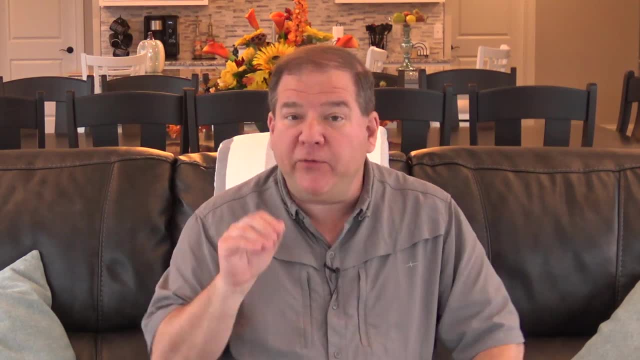 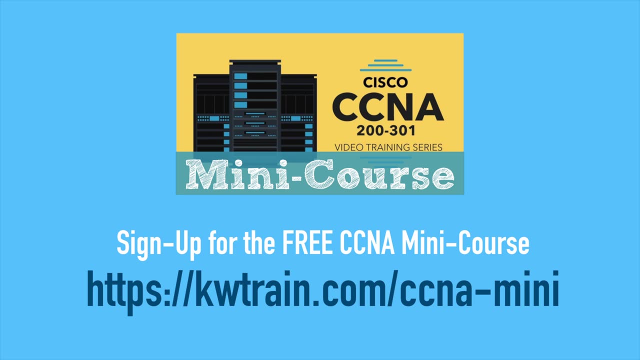 for the series and you're watching it in my portal. but if you're watching this on YouTube, if you want to get the next videos in this series, you've got to go to this link on screen right now. That's going to get you signed up for this CCNA mini course and over the next few days, 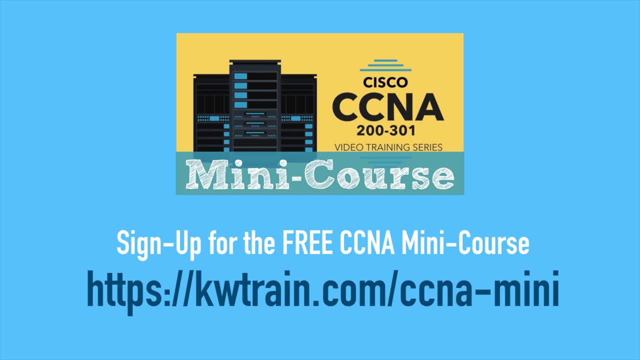 I'm going to be rolling out different videos as part of this course that are not going to appear on YouTube. So if you're watching on YouTube, go over to this link right now and get signed up for the entire mini course. And I want to give you a little bit of information about the QoS training and I'm going to give